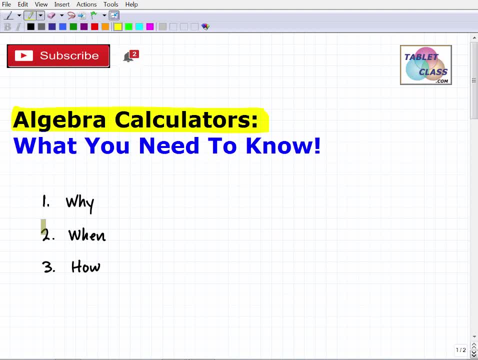 If my teaching style is something that you like. I actually have a full, complete math learning program. I'll leave a link in the description of this video. Also, I literally have hundreds and hundreds of math videos on my YouTube channel. Hopefully you can check those out if you're interested. But let's get right to 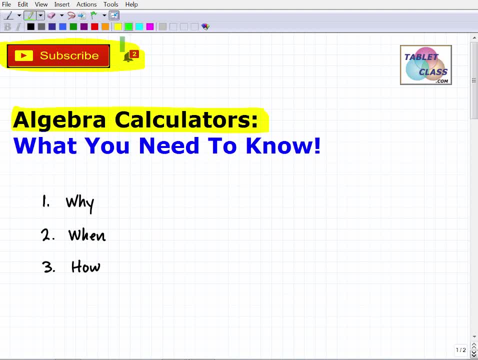 this and talk about algebra calculators. So let's go to our first idea here. So why would you be wanting to use an algebra calculator? Well, a couple ideas here, right? So most students- not all, but most the majority, I would say- and maybe like: 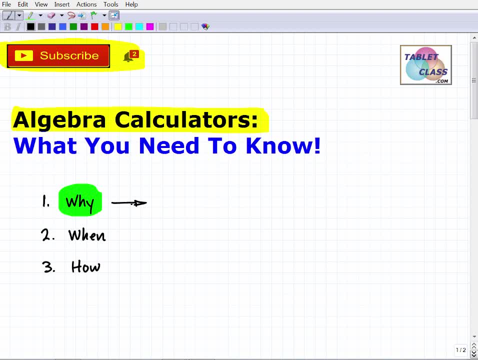 in middle school or high school- especially in, say, high school- are looking for like a shortcut, And I could totally get that. You're like, hey, you know what I don't want to do this math, You know. I just want to like plug stuff into this. 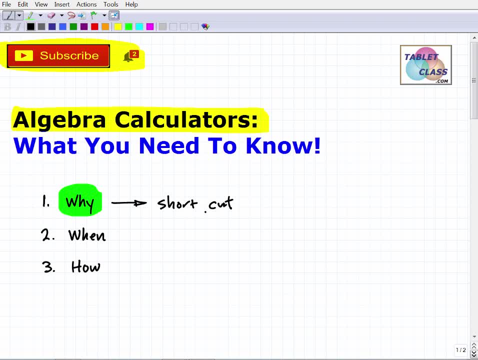 calculator and get my answer. Okay, so that's understandable. Okay, so I can understand. all right, you wanted to take a shortcut, But oftentimes students will use algebra calculators because they don't really know what they're doing. So 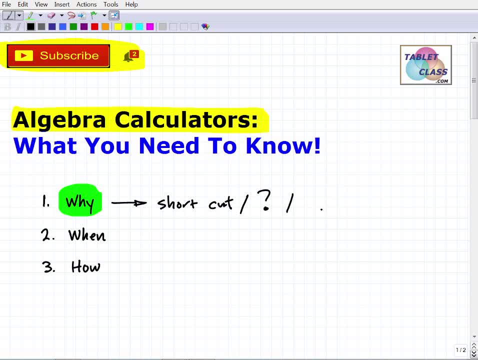 they're like: well, I don't know how to do this particular problem, So I'm just going to type it into this algebra calculator and hope that I'm going to get the right answer. So if you're doing your homework, etc. you know you're going to, you know. 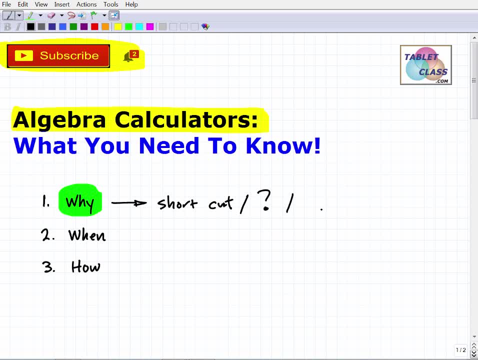 sit there, get your algebra calculator handy and you're going to type everything in. By the way, before we go any further, there's all types of algebra calculators. There's a lot that are online, And then you actually you can. 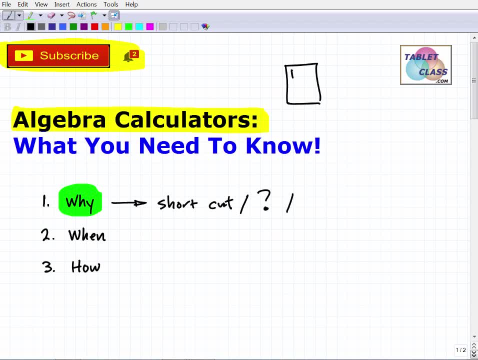 actually in some scientific calculators- you know, I'm kind of trying to sketch one out here, like a TI-83 or TI-84, or. scientific calculators are very advanced. You can actually perform a decent amount of algebra calculations on here And when we're 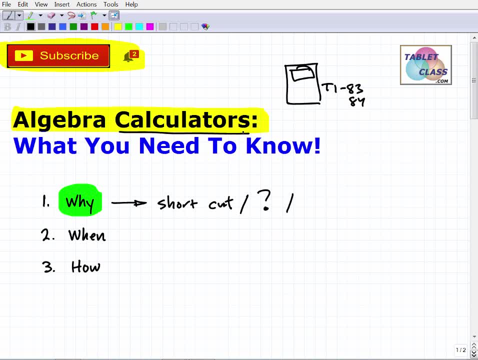 talking about algebra calculators. we're not just talking about a calculator, right, a calculator where you plug in different numbers and whatnot. You're talking about something that could solve an equation, do something algebraically with variables, etc. So even these calculators here- TI-83,, TI-84, there's a lot to do, But again it's. 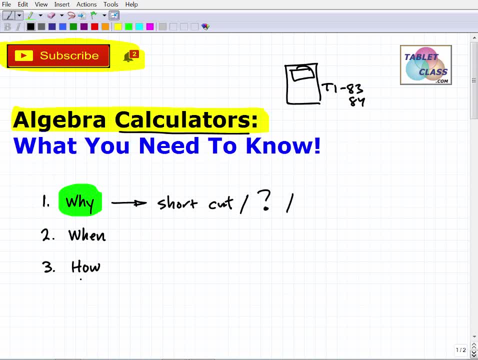 kind of. you know I'm going to kind of get to my next thing how down here in a second. Okay, so we're talking about calculators, we're talking about the whole spectrum of them. There's ones that are way more advanced online, But if 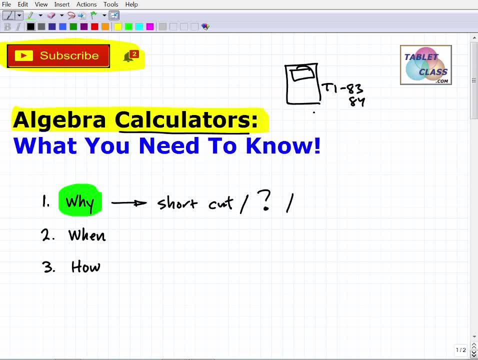 you're walking around with one of these scientific calculators, you might be thinking: well, it's not an algebra calculator. But actually there are some algebra calculations you can do on these calculators. But let's continue on the video. So first thing is why? So you want to take a shortcut, speed up the time. but 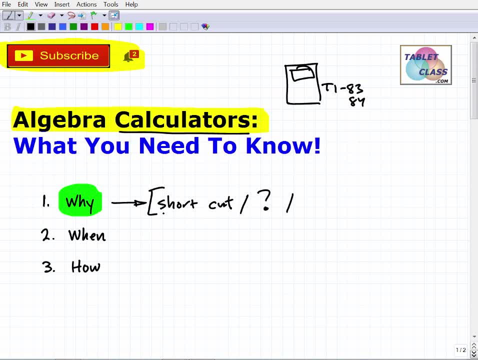 you really don't know what you're doing. I would say this is the majority of people who are interested in using an algebra calculator, right? So I understand. hey look, you want to. you know you want to go faster and you don't know how to do. 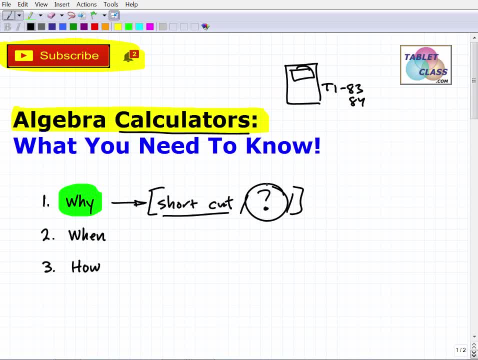 something, you're going to get a tool to help you out and get the answer. Well, I got that, But here's the deal. If this is your reason, you got to be very careful and you don't know how to do something and you're using a calculator to basically. 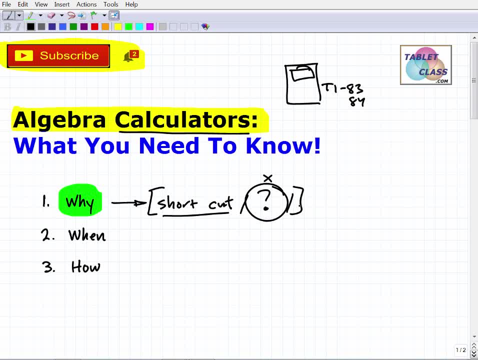 get an answer, but you don't know how to get the answer by yourself. this is a big problem. Okay, so I would say this is probably one of the biggest risks, especially with the shortcut. So if you're using the calculator, just to you. 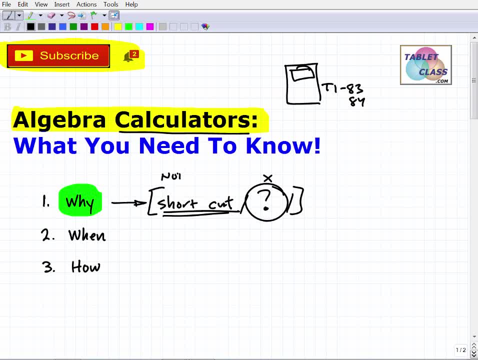 know, speed things up, you're not getting true practice. So here you're not really getting the practice that you need to really understand the math and the problem-solving process. And then if you just basically plug in stuff into a calculator in hopes to get right answer, this is really. you know this. 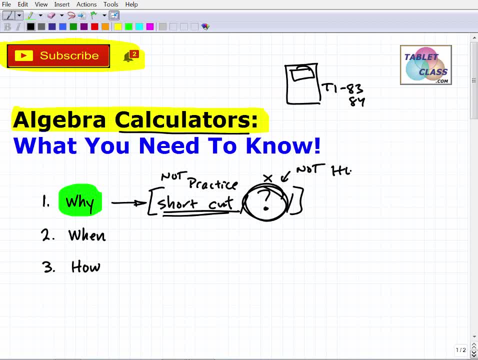 is not helping you, okay, It's not helping Now. you might say: well, it's helping me right now with my homework. Yes, okay, I got that. Maybe you could turn something into your teacher, but it's not going to help you on your test or quiz, So you got to be. 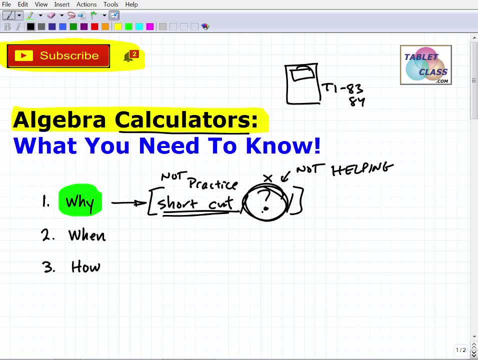 careful, right, If your motivations are you know these two things, then you know you really got to be careful with the calculator because the calculator can really, you know, hurt you. Be better off With actually not having a calculator, because you'd be forced to learn it, You wouldn't have. 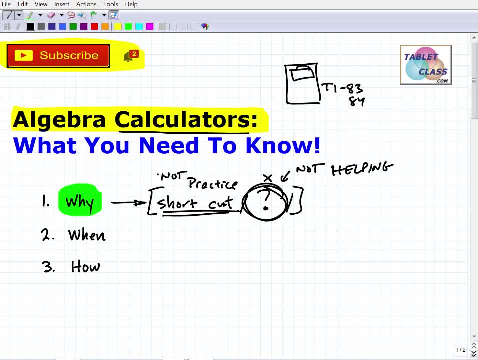 no other option, or you would actually have to sit down and do the problems. as much as you may not want to, It's still going to benefit you in terms of learning math. Now, the last reason here. you know there could be other reasons, but the last reason is to use it. 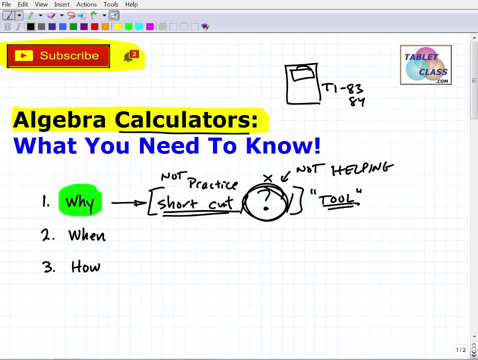 as a tool, And this is really the ideal kind of scenario: that you're using the calculator as a tool, An assistance right, Like something to double check your work, like, or to you know you can be, you know, do one problem by hand. 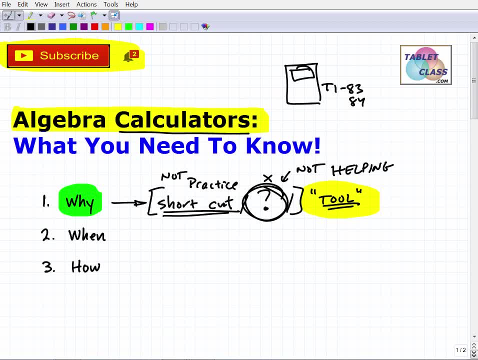 and then you know, plug another one into the calculator and you kind of know what's going on. You think you know how the calculator is thinking because you could generate the answer by yourself. So if you're using it as a tool, a calculation tool, then that's. 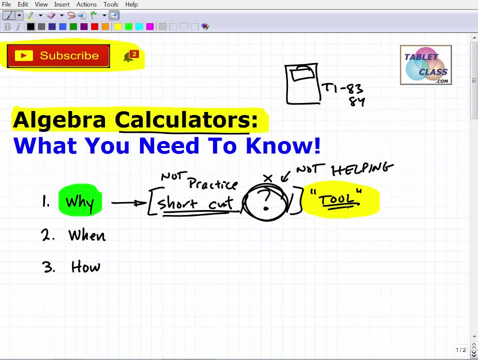 that's good, Okay. So calculators, you know, for me as a math teacher, they're important, Okay, They're definitely an important part of your your math learning. Okay, And especially in algebra, you really do need calculators. but you've got to look that, look at them as. 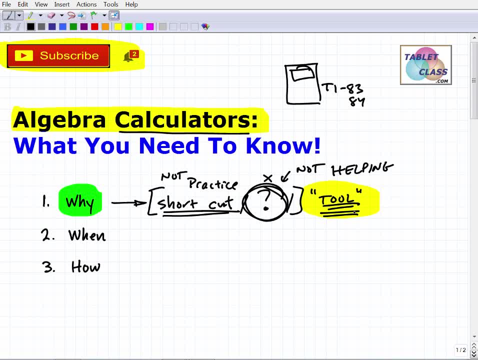 a tool, like a support tool, not a replacement, to actually do problems and you don't. when you can't do them or you know, you want to just kind of just replace, you know doing the work by a calculator. Now I will say this much: Once you learn the material, let's. 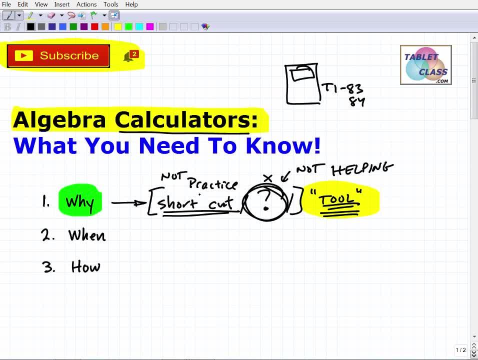 say: you're a, you know, a scientist or an engineer, and you know, and you could plug in and use calculators to get your answers and you're perfect. But if you're in a professional profession, then that's completely different because, like 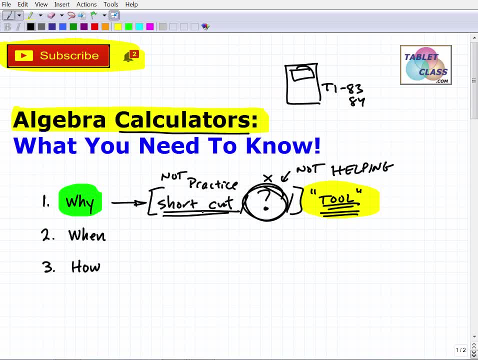 engineers, they have to learn a lot, a lot of math, but they don't do everything by hand like calculus or whatever They have, you know computer programs and stuff that run, but they understand the math behind it. Okay, Again a tool, especially if you're learning. 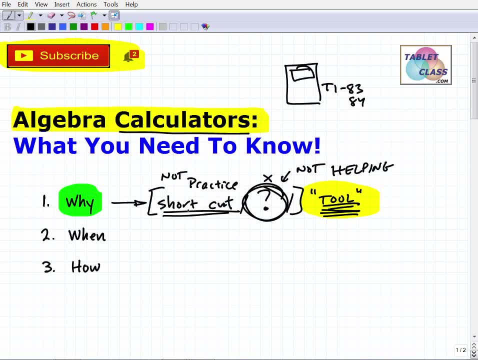 you got to be careful with calculators, but I think I probably um kind of harped on this enough, So let's move on. Listen. the reason why I'm making this video is because I don't want you to, you know, become dependent on algebra calculators. 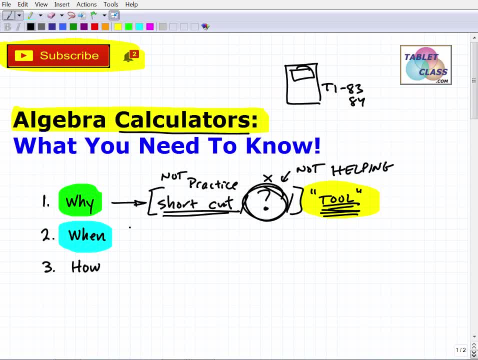 That's really you know. they're not going to serve you well later, later down the line in math. Okay, So when should you use a calculator? Well, this is something that you should really try to get guidance, uh, with from your teacher. Okay, Now, your teacher should probably in. 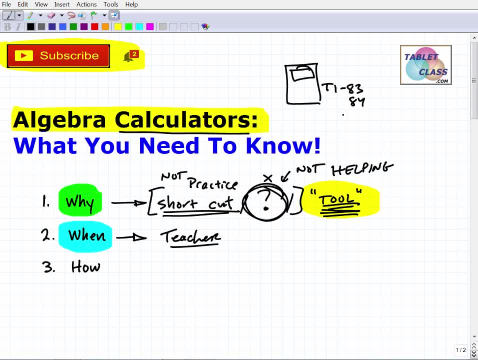 your class say: here, you know, I'd like you to have a particular type of calculator, um, you know, for this course. So get some guidelines. because here's the thing: if you're going in and taking a test, all right, and you could have your handheld calculator, they're likely. 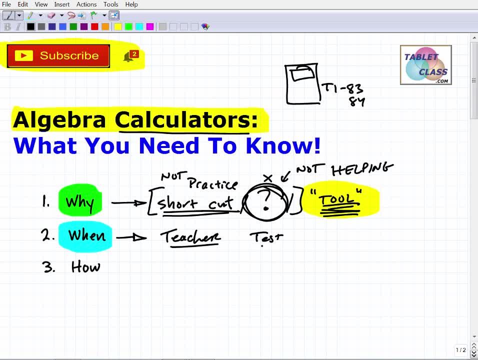 not going to let you do that. If you use your cell phone calculator, they're definitely probably not gonna let you go online and use an online calculator. So know from your teacher, kind of like, what type of calculator you can use. Now, we're not, we are talking about algebra calculators here, so you may. 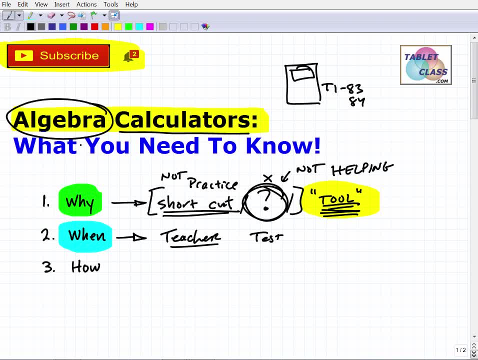 not be able to use any type of algebra, algebra calculator- Okay, On your, on your exam or quizzes. So again it goes back to the practice thing. You want to be smart? Okay, You want to make sure you can do the Brahms. um, that you know your teacher, your your teacher. 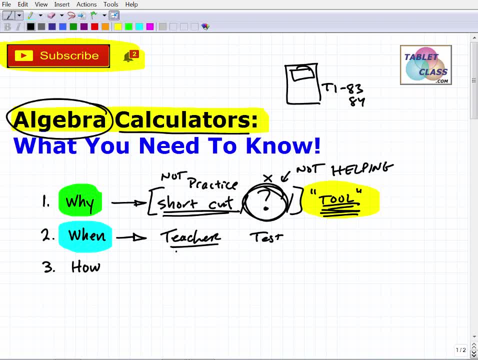 is stating that's going to be on a test or quiz. So if you're not quite sure, simply just ask them. raise your hand, say Hey, can you know what's the guideline on on calculators, uh, et cetera. But again, this should have been pretty, pretty clear now when you should. 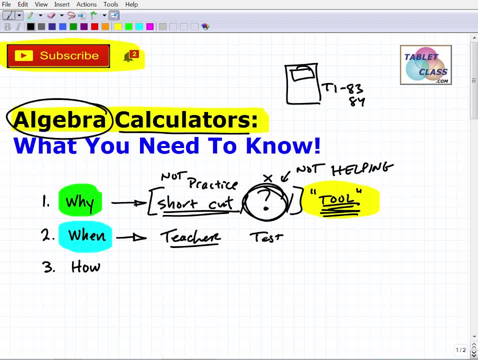 use them. Okay, Even if you got. uh, your teacher says no, you can't use an algebra calculator test. Again, I think if you're kind of studying or maybe doing your homework, study for a test and use it as a support tool just to double check some answers and whatnot. 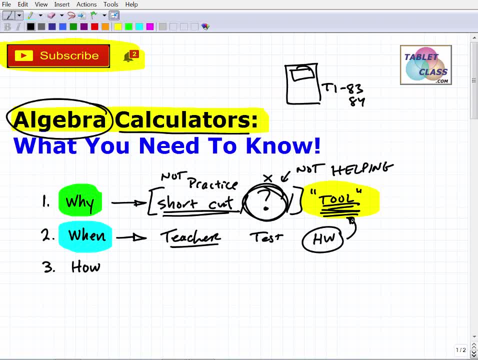 I think that's perfectly, uh, okay, Okay. Again, it's a, it's a tool, it's a support tool for you to be learning algebra without the assistance of a calculator. Um, now I will say this, uh to um. as you know, nice as algebra calculators are, they do have their 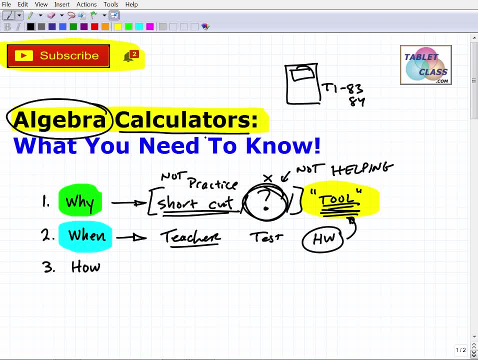 limitations. There's some things, and of course there could be some very, very advanced algebra calculators out there, but there are things out there that probably the calculator, a calculator, is going to be difficult to program in order to get the answer, uh, to the question. 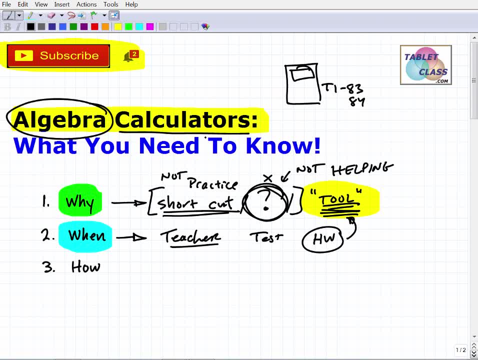 Okay, Various type of type of uh scenarios et cetera. I don't want to get into it because there's so many facets of algebra, but when we're talking about solving equations or inequality, or graphing lines or multiplying matrices or solving a quadratic equation, yes, a calculator. 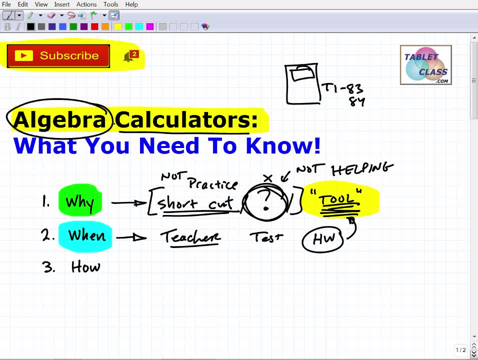 can definitely help you out, because it's kind of plug and chug: You just plug in the values and you got your variables there and you kind of go. but conceptually to be able to- you know um- answer questions that are a little bit more. you know abstract, you know it's. 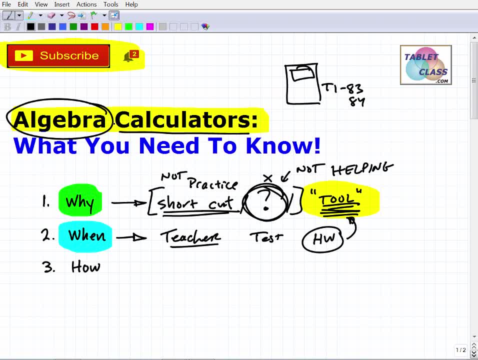 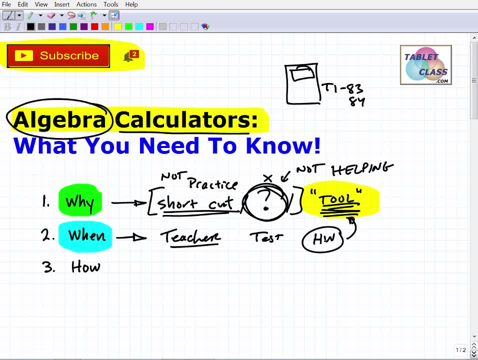 a little bit more, you know, based uh, or directed towards getting solvent, a support for a particular solution or graphing a line. those types of things probably really, really, really going to get the most help from an algebra calculator. Okay, So let's talk about. 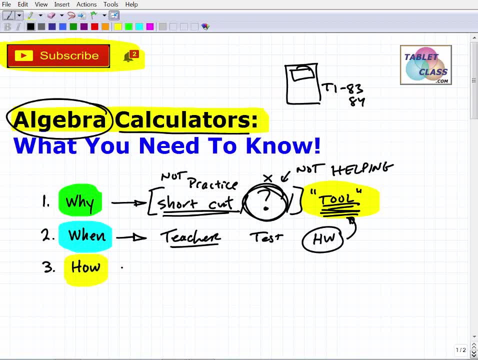 my last uh item here and that's how well I can tell you right now this is a huge thing, even with a regular calculator. okay, a lot of students don't know how to even use their basic scientific calculator because, remember, a calculator is just. 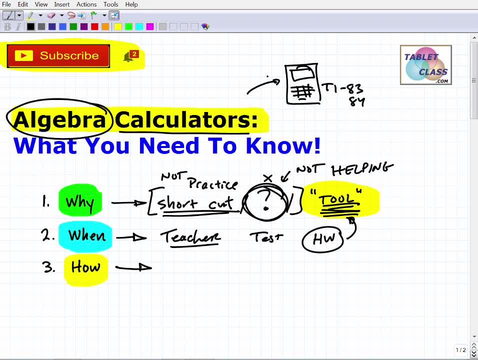 again a tool, what you plug into it. if you, if you type into your calculator, you know whatever. if you don't do this correctly, if you don't plug in the steps correctly in your calculator, you're gonna get the wrong answer. so again, you need to understand the math to be able to talk to your calculator appropriately. 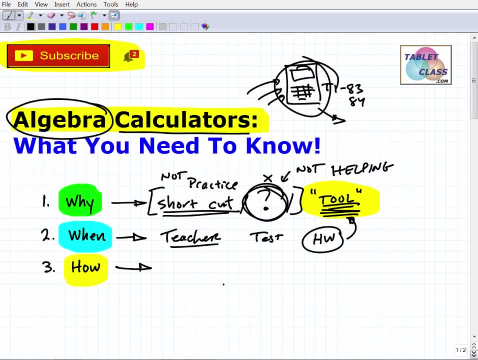 so let me give you an example here. let's say, I was trying to figure out with 2 to the- let's see here, let's make it more interesting- 16 to the 2 thirds power. okay, now, this is an algebra, but I'm going to give you a good example here. 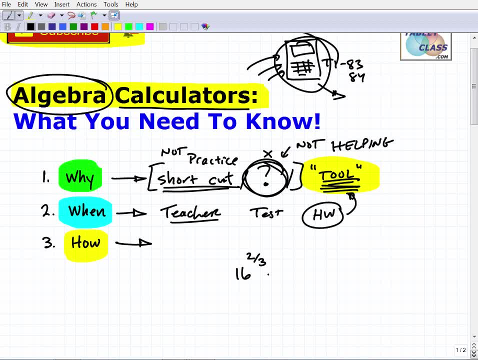 okay, so 16 to the 2 thirds power. now, if you were, you know, in an algebra course, you would be okay, you would be able to simplify this using radicals, and then you can kind of, you know, go from there and kind of do the work. but let's say 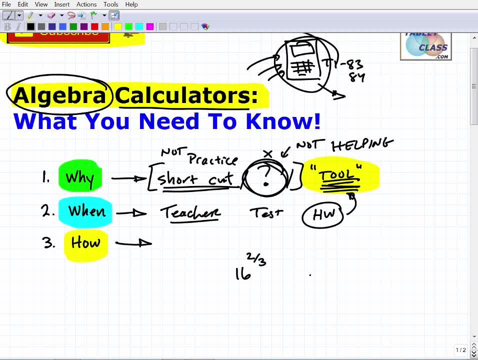 you wanted to kind of get an answer for it and you went into your calculators. okay, I want to go ahead and go 16 to the 2 thirds power. now again, this is I'm just talking about calculator mistakes and when you're using an algebra. 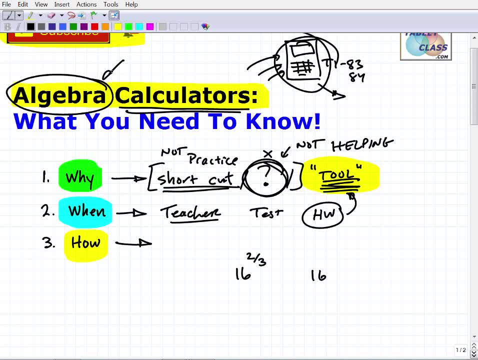 calculator, it gets that much worse, okay, so, in terms of not knowing what you're doing, you're gonna get a wrong answer. you remember that the calculator is always going to give you some answer, but it could be wrong. so a lot of times the students don't know what they're doing and they don't know what they're doing. 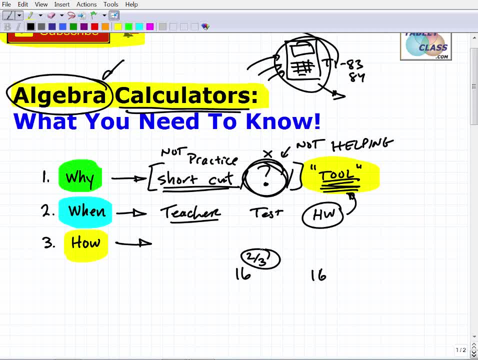 so you might want to go back to this and look at this and say, okay, let's see what's happening here. now let's go back to this, we'll go. okay, let's see, this is 16. now I'll take this to a power, right? so if I have 2 cubed and most calculators, 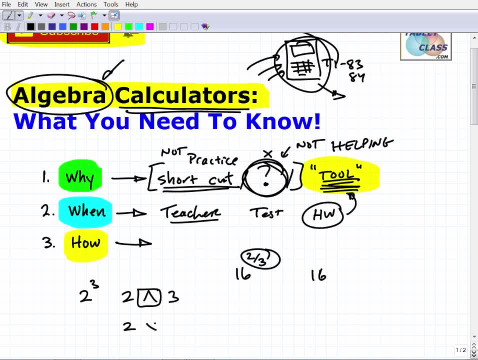 you have a button that's like this: 2 to the 3rd power, what we call a little carrot. another button might be like this: X to the y to the third, or 2 to the y to the X. usually it's one of these buttons that expresses a power or an exponent. so 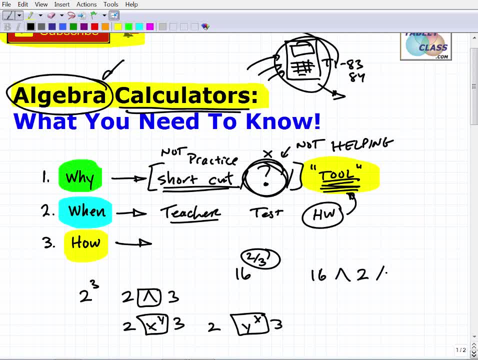 to the two divided by three, power. okay, he said I did here. so when it goes you're gonna say okay, sixteen to the two-thirds power, you'll? you go, you type into your calculator sixteen and you hit the little button here which is for the exponent and you plug in two-thirds, okay. so what's the matter with that? you're. 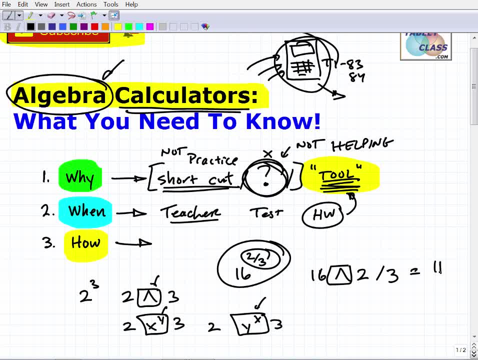 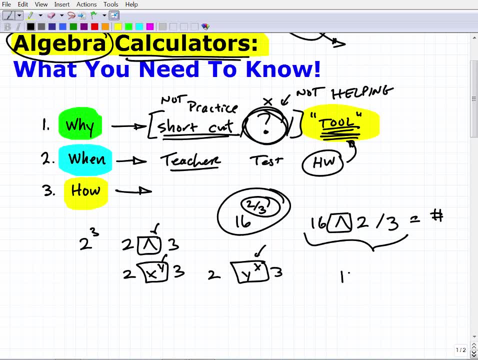 thinking that you're gonna get the right answer. you hit enter and you get some number. well, what this? your calculator is interpreting this right here. it's thinking this: that's a sixteen squared divided by three. your calculator is looking at it like this: sixteen squared divided by three, and you're gonna get. 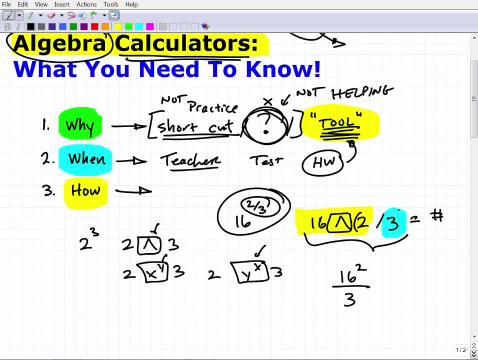 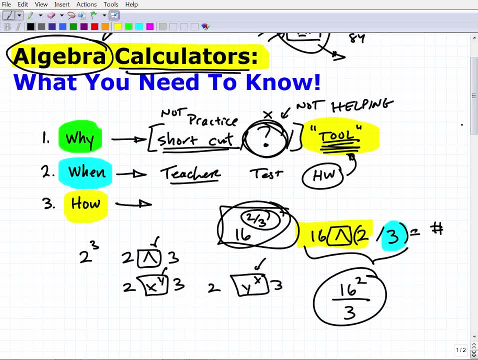 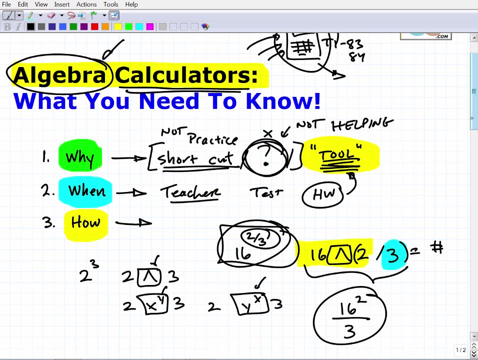 the wrong answer, because you don't realize that you really need to put this in grouping symbols. all right, to get what you really want, which is this, not this. so this is this one of the main major um. there's so many examples of students using our calculator to try to to get an. 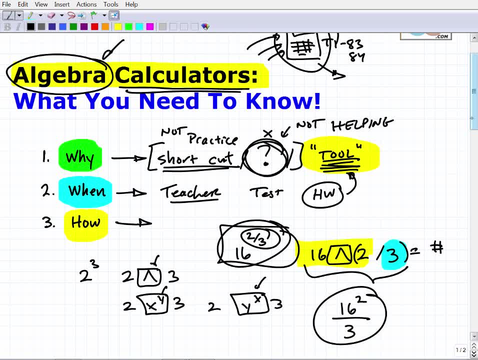 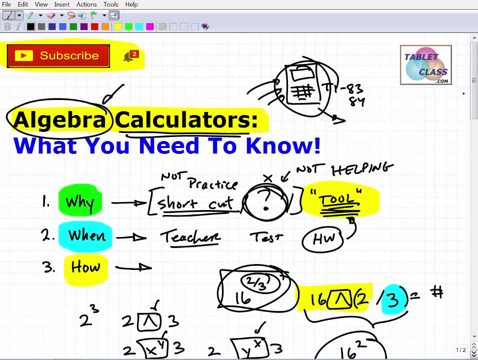 answer. and then they, you know, because they don't understand the math behind it, it's you know they're getting the wrong answer. so again, just because you have an algebra calculator and you'll be able to do things, and you're like, okay, look, I'm getting all right. you know, I'm getting something out of it doesn't mean that.